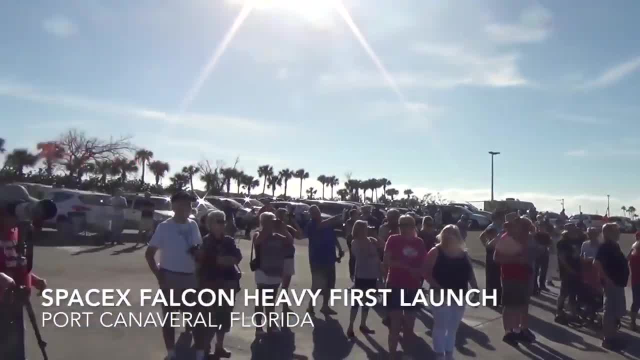 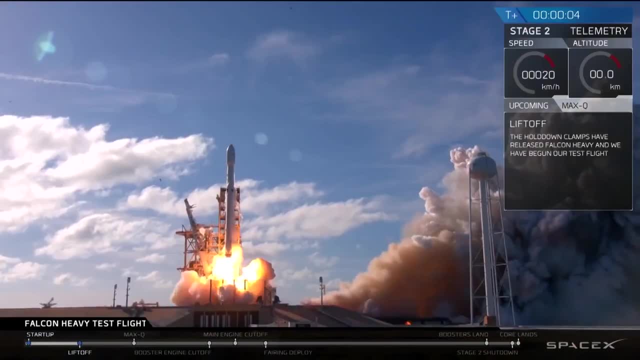 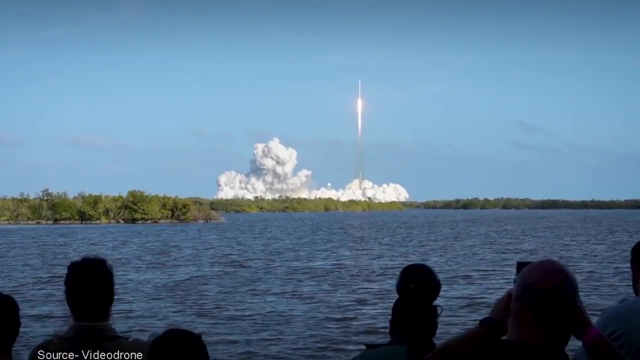 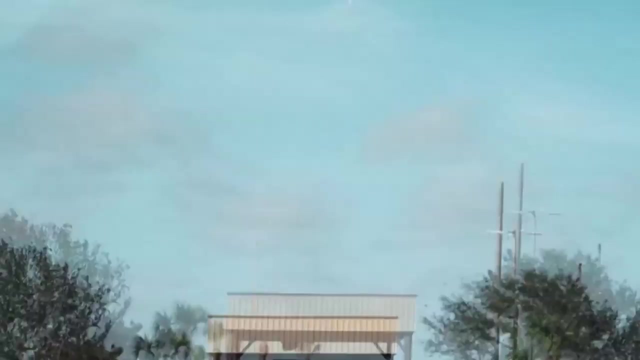 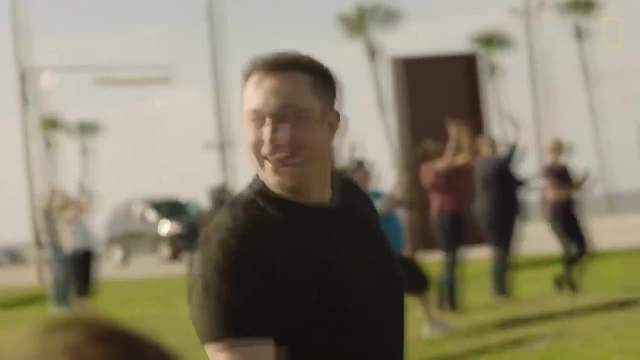 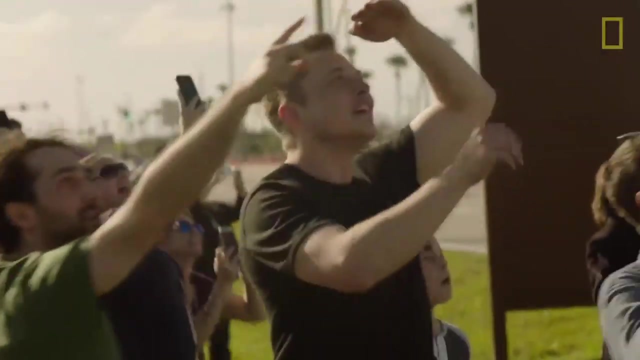 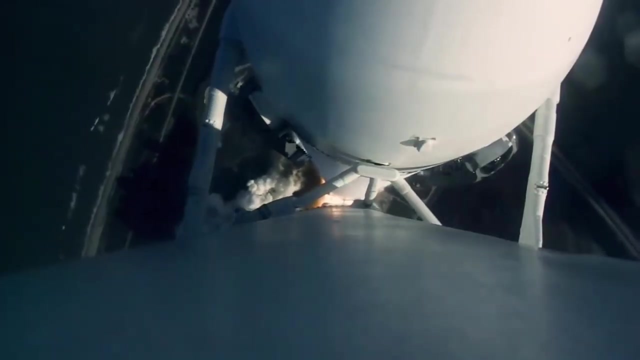 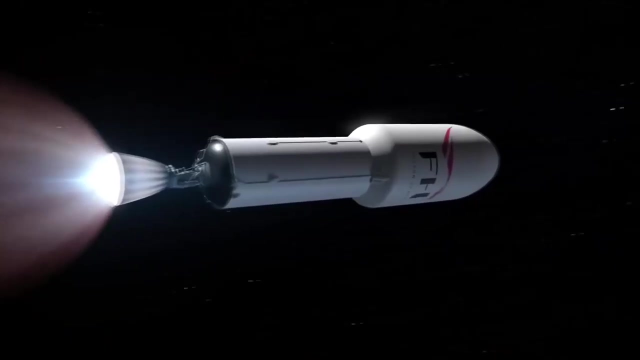 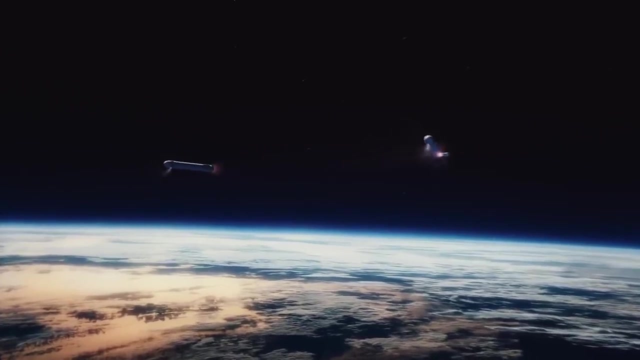 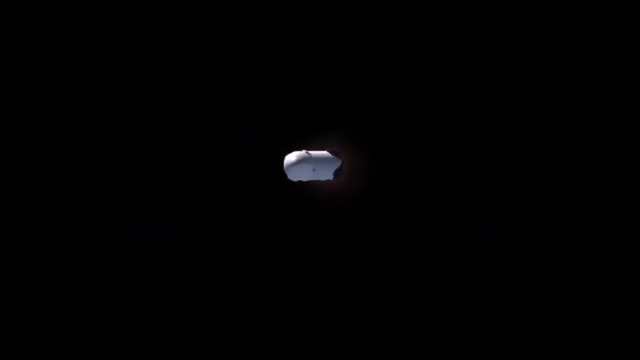 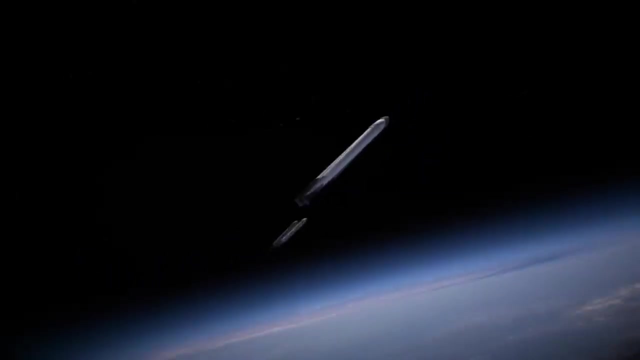 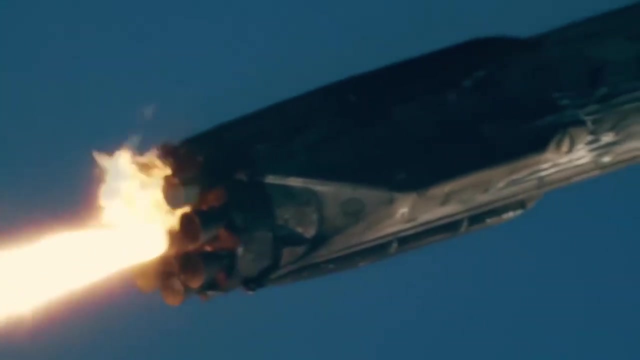 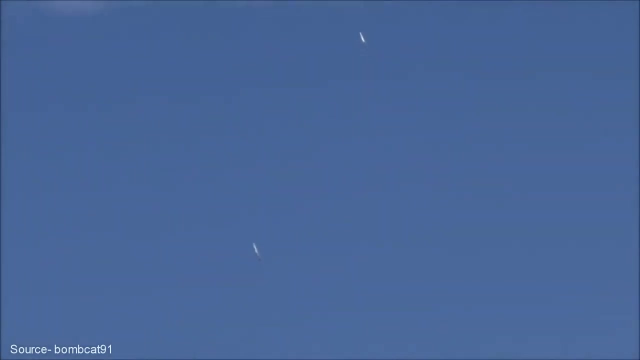 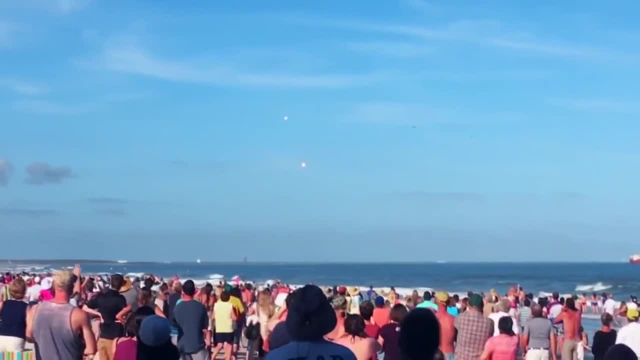 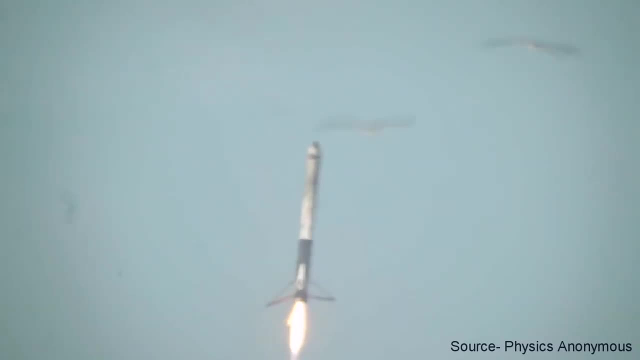 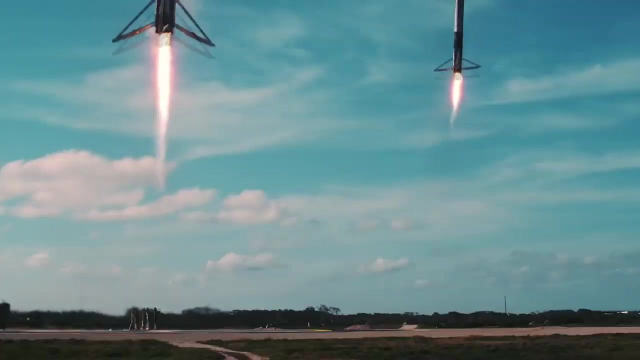 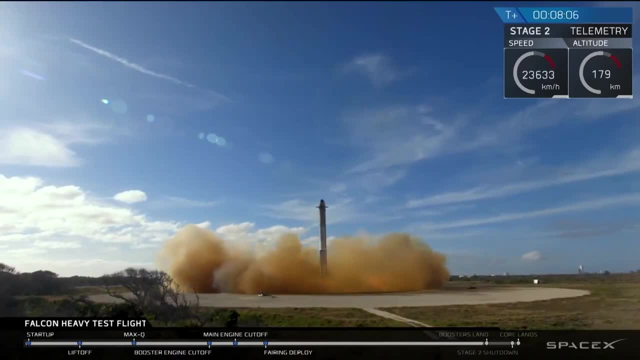 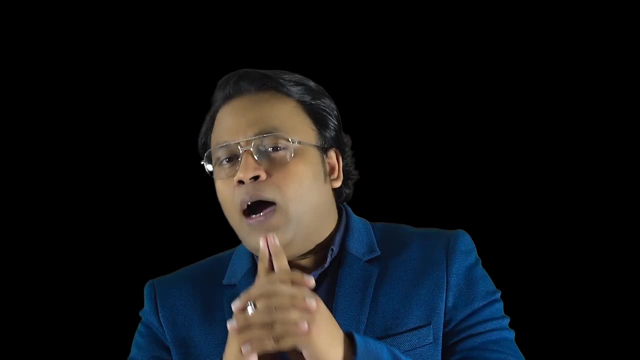 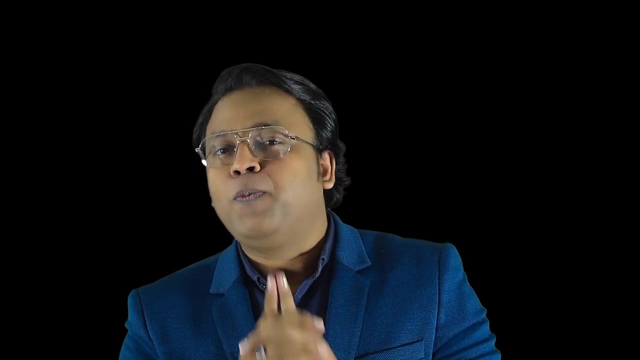 precisely on a target at Cape Canaveral. What you may be wondering is: how did it do that? How did it do that? How did it do that? Well, out of the million things used, one of the most important things used is trigonometry. 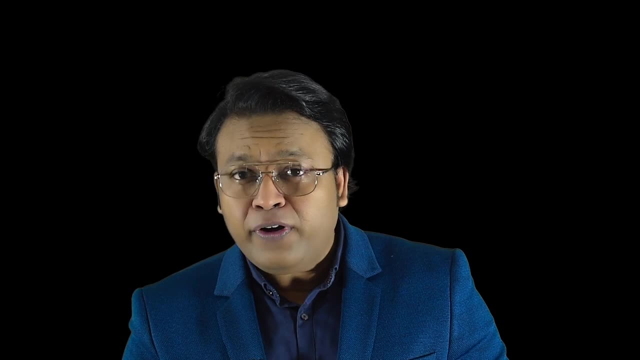 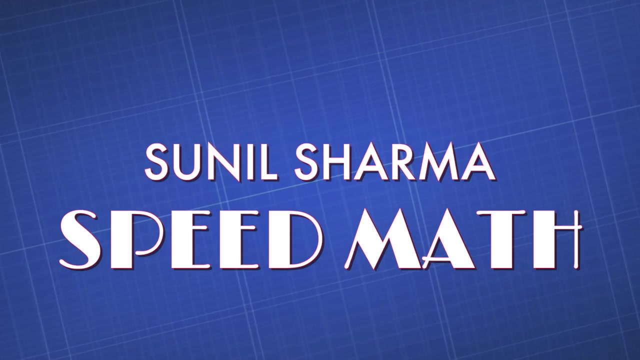 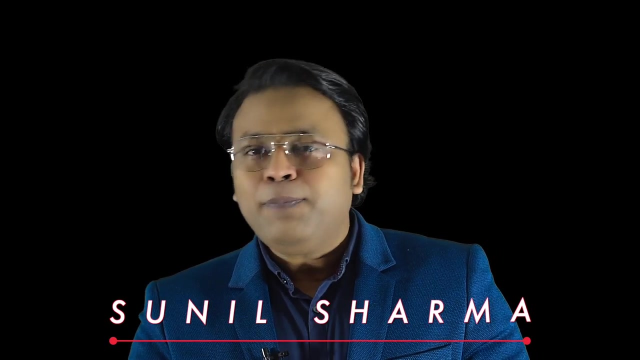 to plot the trajectory of the path. Oh so, do you find trigonometry difficult, Guys? welcome back to my channel, Speed Math, where you'll find a lot of stuff related to maths. I am your mentor, Sunil Sharma, and in today's video we are going to discuss why trigonometry 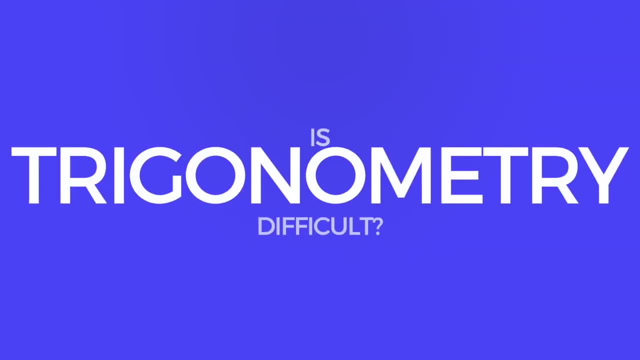 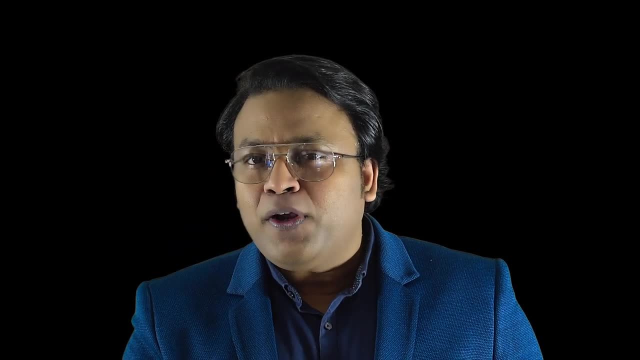 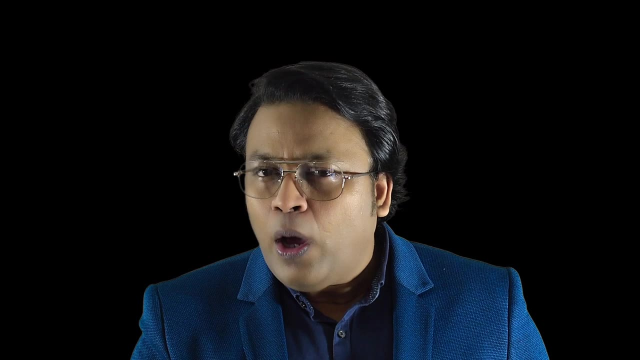 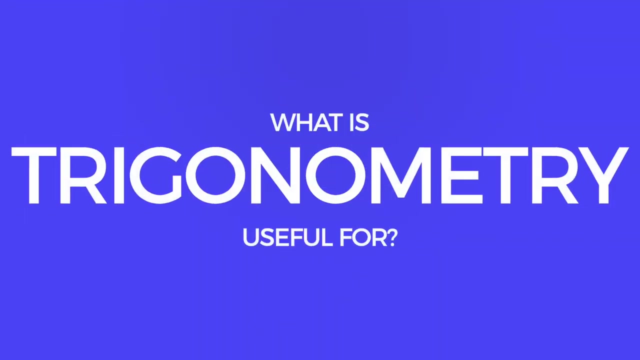 is very, very important. Trigonometry isn't difficult. If it seems difficult, that's because you were taught in a manner that doesn't work for you. Different people learn in different ways, but sometimes you are taught in one way as per your teacher, whereas the way you should be taught needs to be the way you learn. 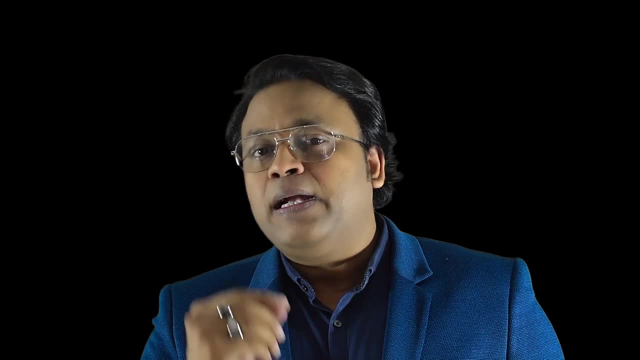 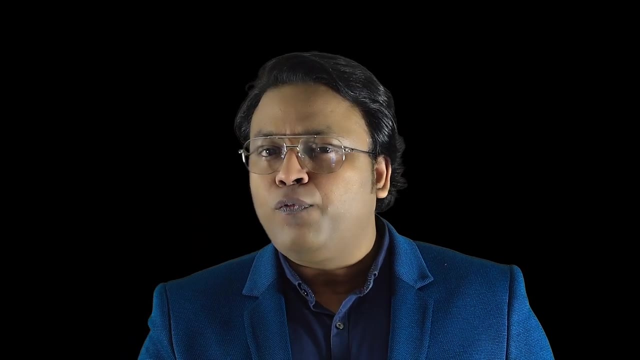 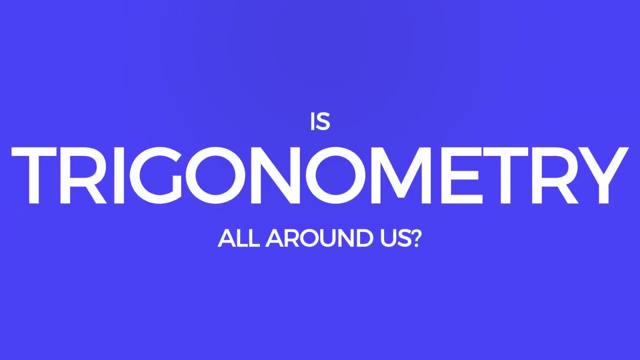 One of the main things that need to be taught. when you learn something is what it's supposed to be good for and what you need it for. If that wasn't part of what you've learned, then that is probably why you don't understand it in the first place. 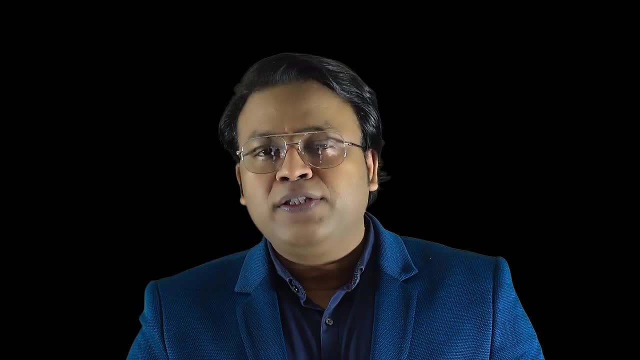 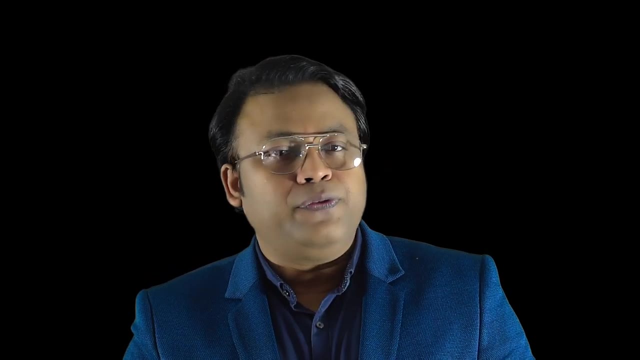 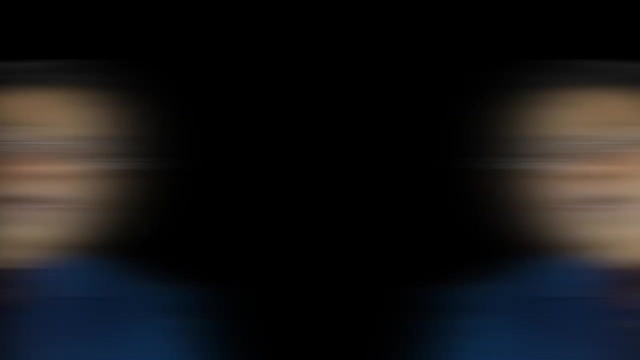 The reason why trigonometry is so important lies all around us every day, although most of us are blissfully unaware of what trigonometry does for us in our lives. It would not be possible to build a car without trigonometry. The homes we live in are built using trigonometry. 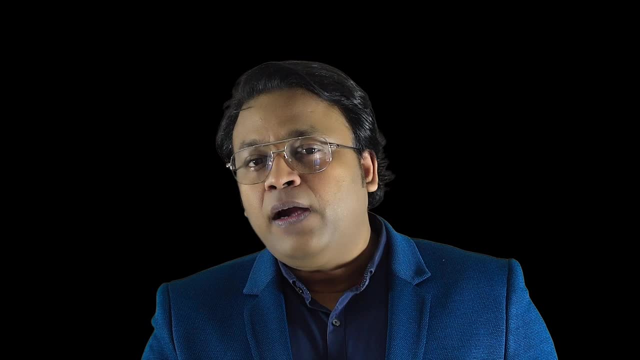 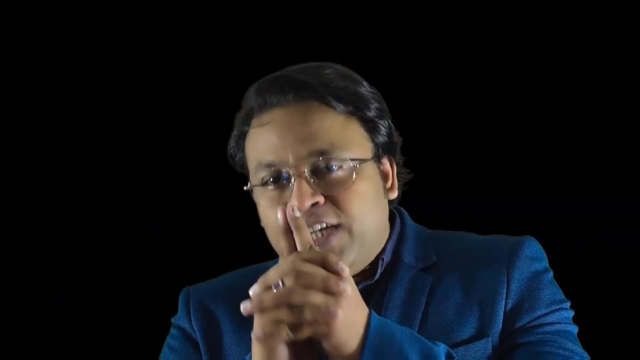 Just about every piece of technology we take for granted is researched, developed and manufactured based on some trigonometric knowledge somewhere along the line. The internet, which has become next to a roti kaptaan makaan, is also due to trigonometry. 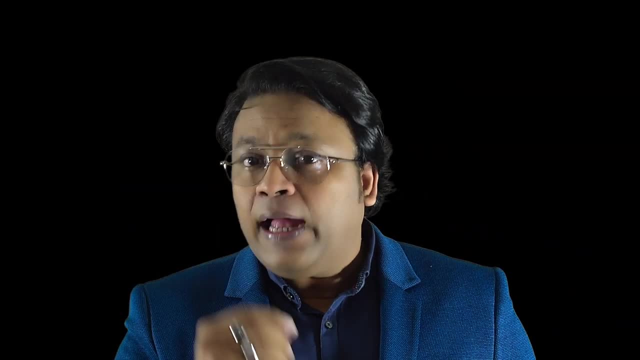 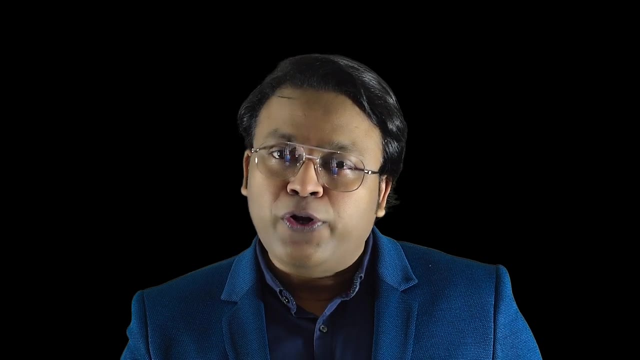 We need trigonometry to launch a satellite, and for that we need to compute launch trajectories, orbital trajectories and re-entry trajectories. Thanks to our knowledge of trigonometry, we were able to launch satellites, and because of which we are now able to launch the world's largest rocket launchers. 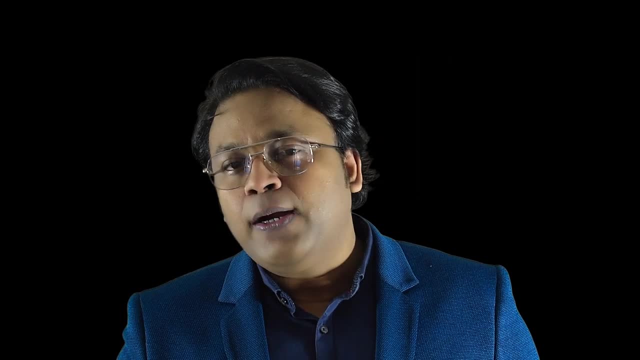 If you want to continue learning more about trigonometry, we are going to tell you how to do it. There are a few things you need to know about trigonometry, such as Google Maps, internet mobile towers, TTH channels and not to forget all social apps like Instagram, FB, TikTok. 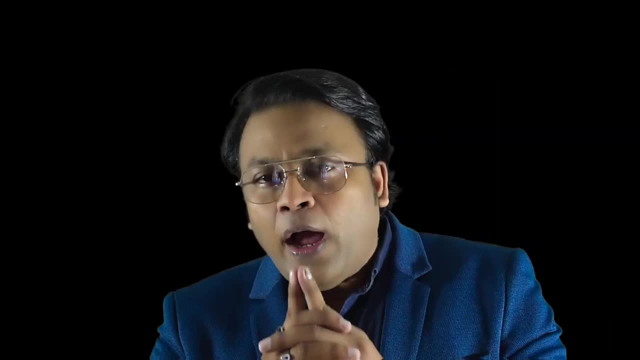 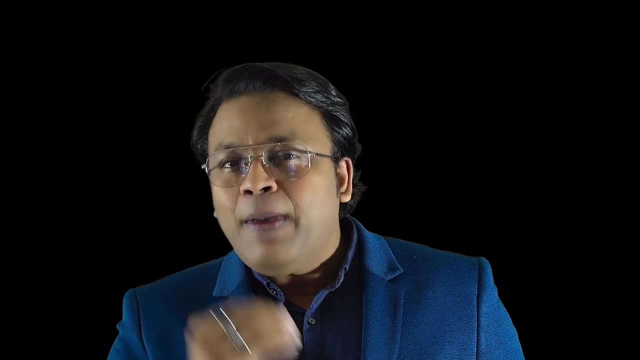 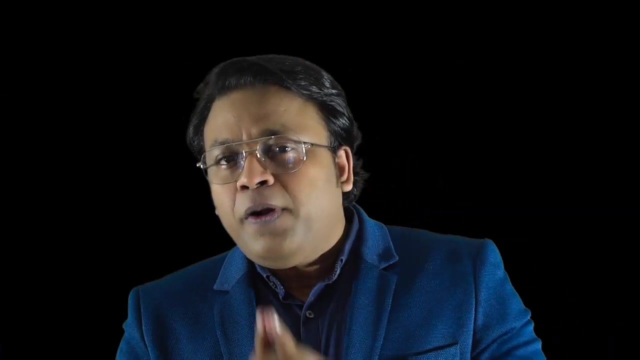 YouTube we enjoy today is all because of trigonometry. Why? because all these apps works on internet, and without internet, all these apps has absolutely no value. Imagine life without internet today. Much of our knowledge about waves, sounds, light water, etc. comes from trigonometry. 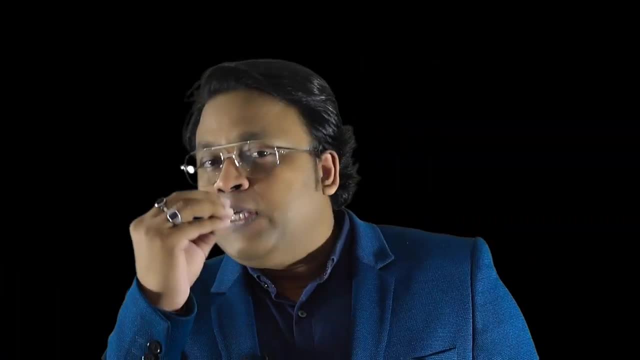 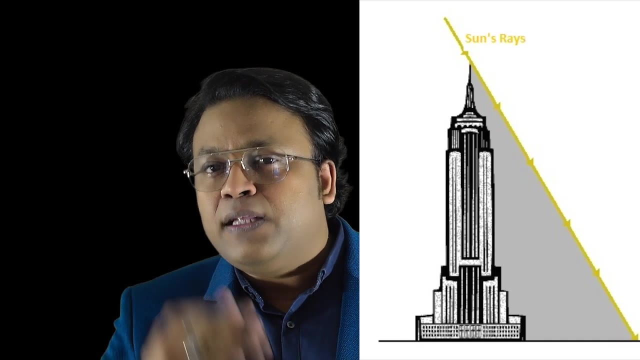 Trigonometry is necessary anytime there is an angle involved: angle of the sun, the angle of the cue ball in a game of pool, or anytime you have to compare two non-parallel lines, like the height of the building and the height of its shadow. 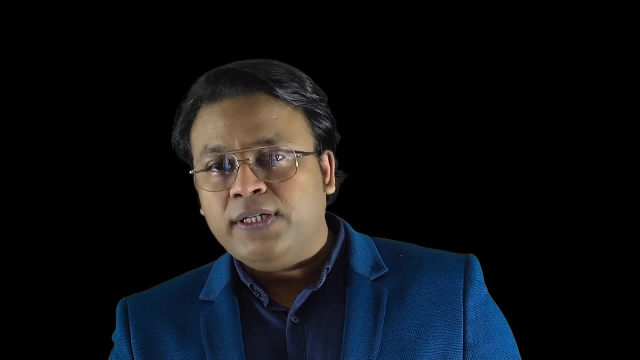 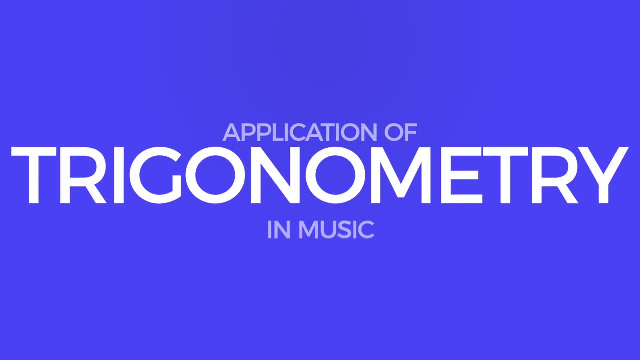 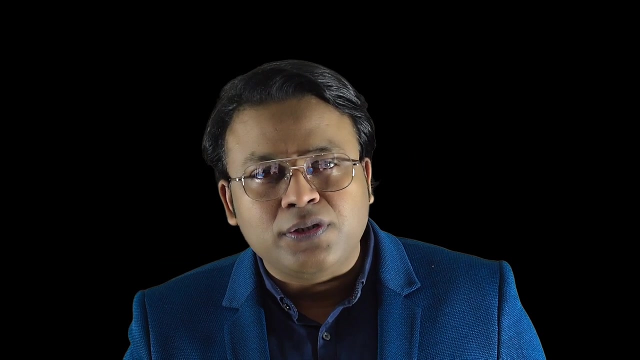 the distance a train is from the crossing and the distance a car is from the crossing. These kinds of problems cannot be easily solved without Trignometry. Sound waves travel in a repeating wave pattern which can be represented graphically by sine and cosine functions. 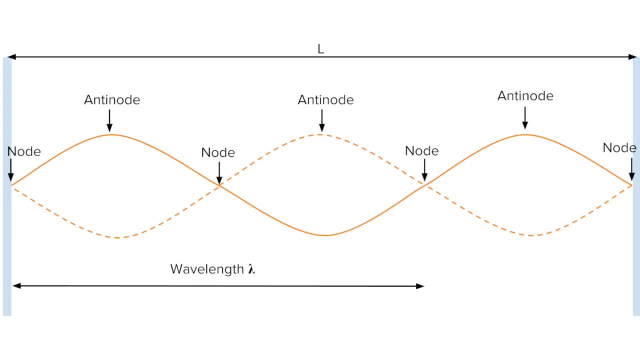 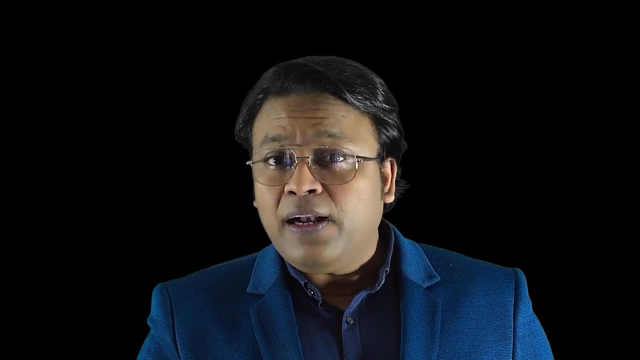 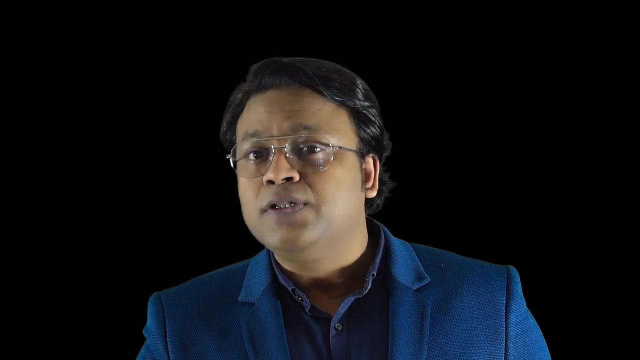 A single note can be modeled on a sine curve, and a chord can be modeled with multiple sine curves used in conjunction with one another. A graphical representation of music allows computers to create and understand sounds. It also allows sound engineers to visualize sound waves so that they can adjust volume. 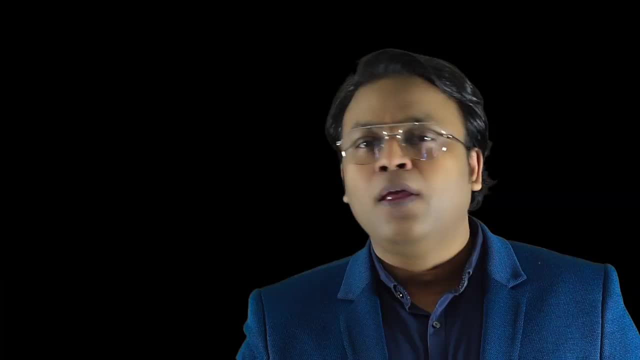 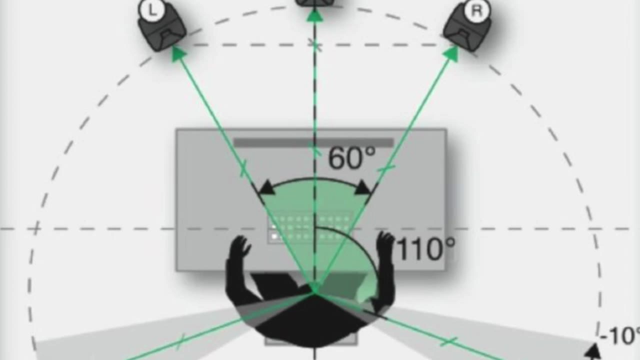 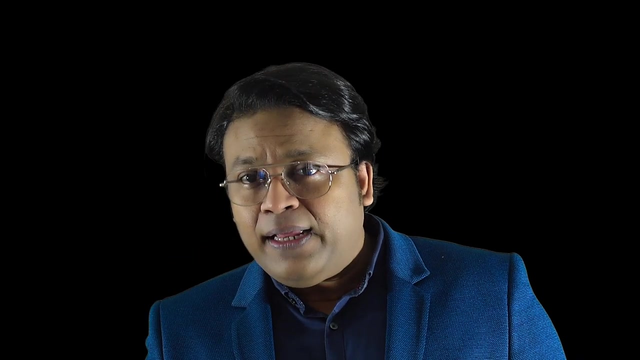 pitch and other elements to create the desired sound effects. Trignometry plays an important role in speaker placement as well, Since the angles of sound waves hitting the ears can influence the sound quality. Modern power companies use alternating current to send electricity over long-distance wires. 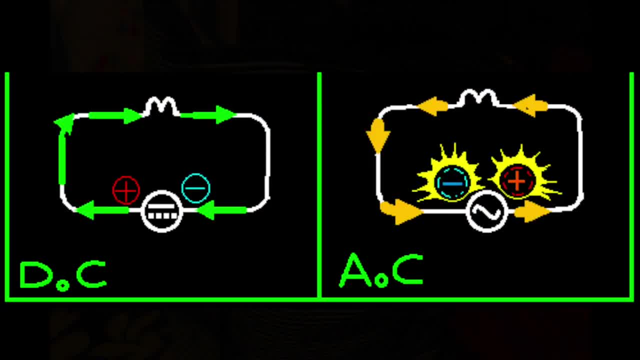 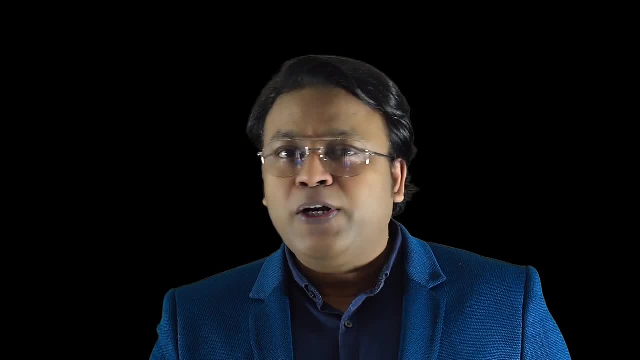 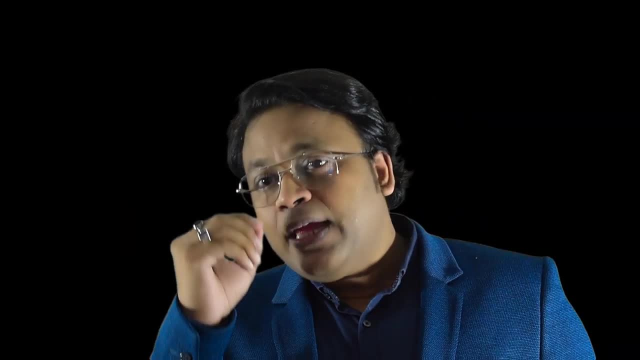 In an alternating current, the electrical charge regularly reverses direction. to deliver power safely and reliably to homes and businesses, Electrical engineers use Trignometry to model this flow and the change of direction. with the sine function, ear and sound waves. It can be used to model voltage. 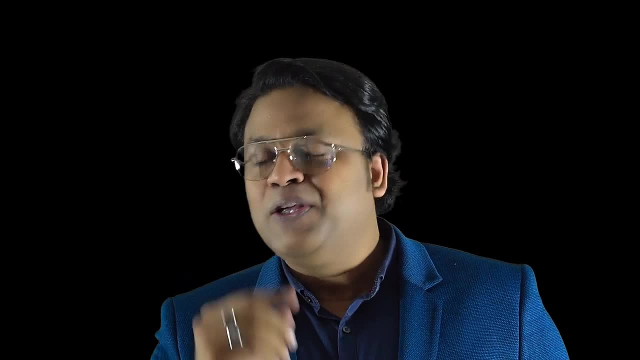 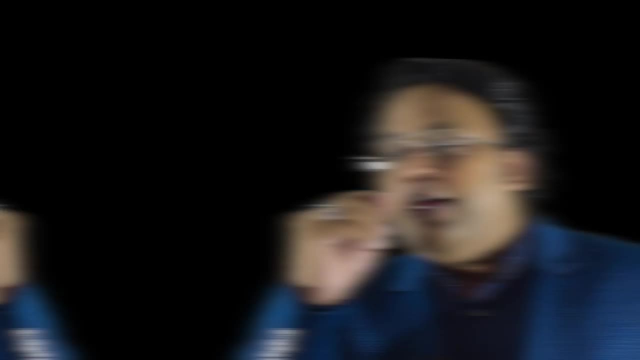 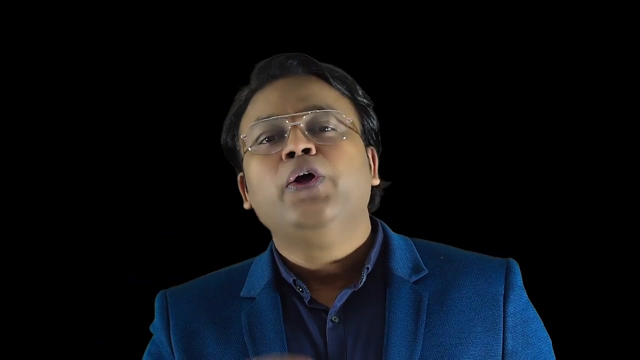 Every time you flip on a light switch or turn on the television, you are benefiting from one of the Trignometry's many uses. Engineers rely on Trignometric relationships to determine the size and the angles of mechanical parts used in machinery tools and equipment. 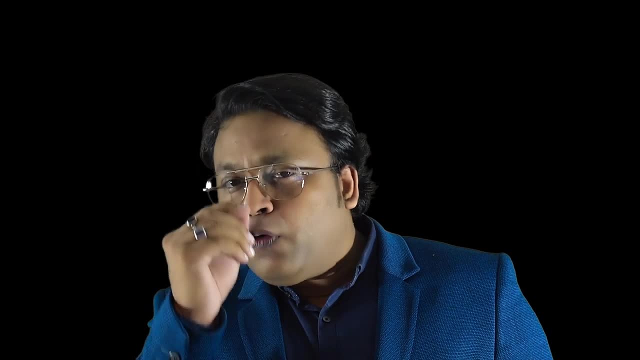 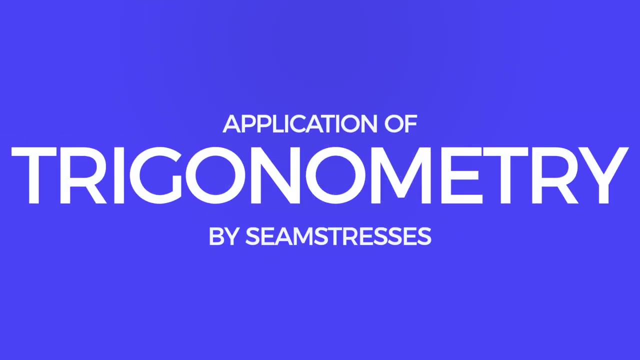 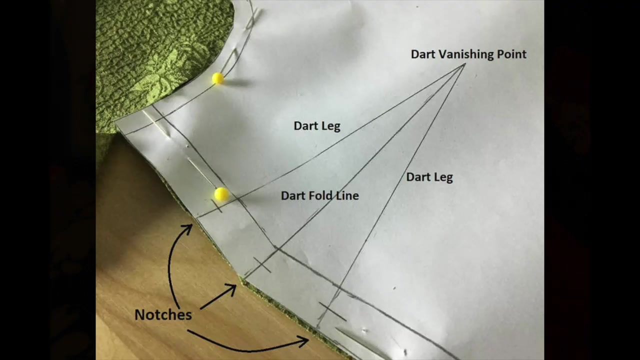 This math plays a major role in automotive engineering, allowing car companies to size each part correctly. Trignometry is also used by seamstresses, where determining the angle of darts or length of fabric needed to craft a certain shape of skirt or shirt is accomplished using basic. 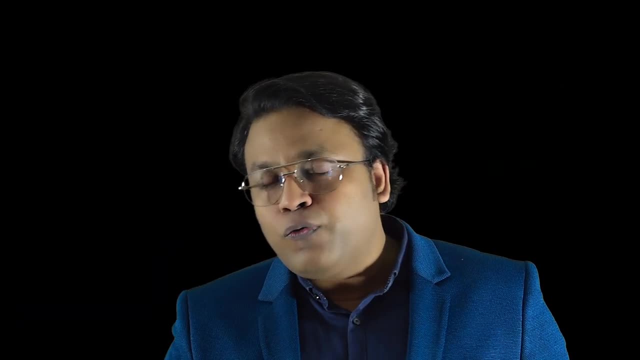 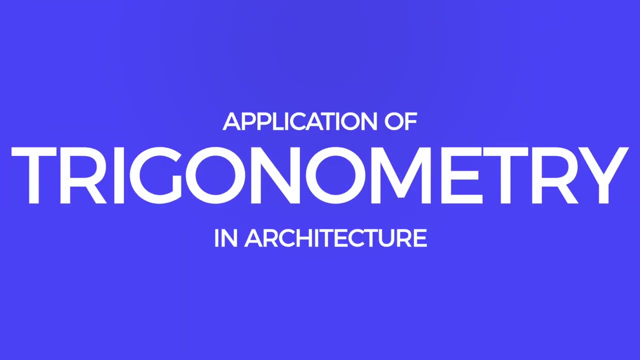 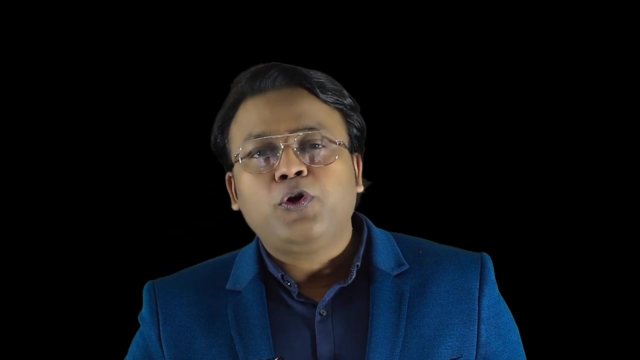 Trignometric relationships. So next time when you are using different designs of clothes, remember those shapes are cut using Trignometric relationships. 3. Trignometric relationships, 4. Perfectlyiary, 5. Tense and Prpayers. 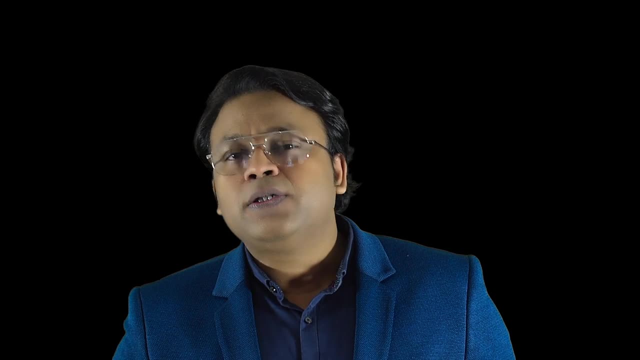 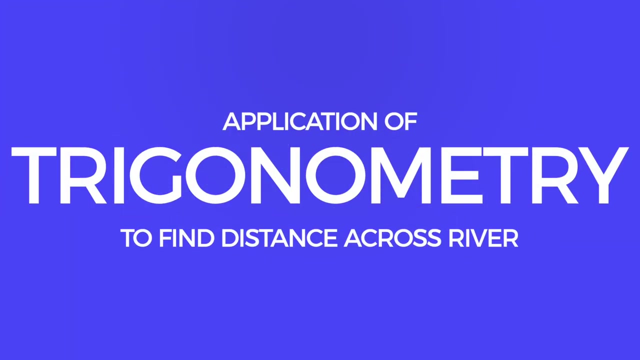 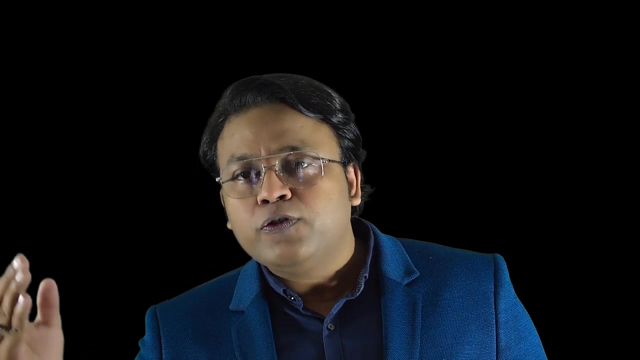 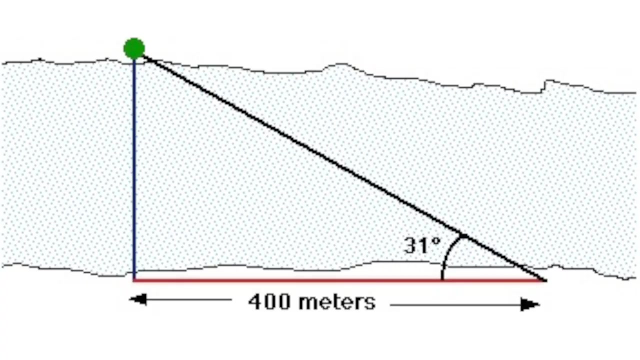 6. Manufacturing, 7. Evolutionary. 6. Architecture, 7. Elevated. 8. Measurement, 10. изв Continue, Delay Fast. 11. íem from some landmark, let's say a tree. Then we head downstream a distance that we can measure. 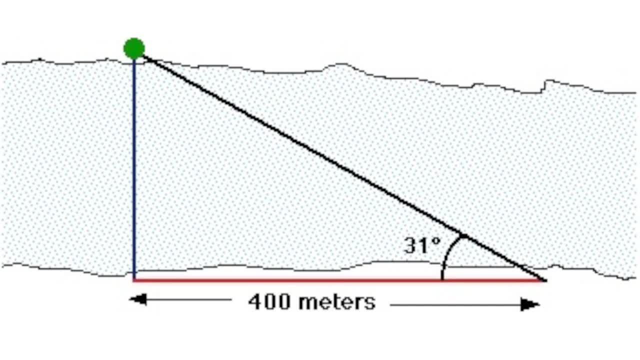 In this case. let's say the distance is 400 meters. That's the red horizontal line in our drawing. Now we take a sighting on the tree from downstream. That's the black line in the drawing. The surveying instrument will tell us. 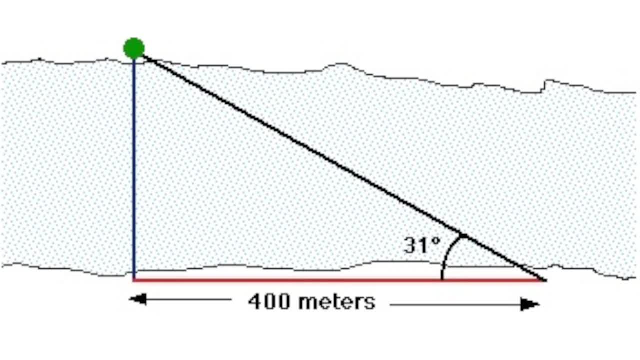 what our sighting angle is. In this case, let's say the sighting angle is 31 degrees. The tangent of 31 degree is equal to the length of the blue line divided by the length of the red line. So if you multiply the tangent of 31 degrees by 400 meters, 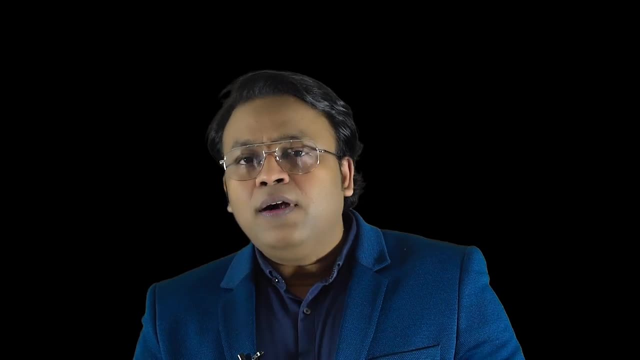 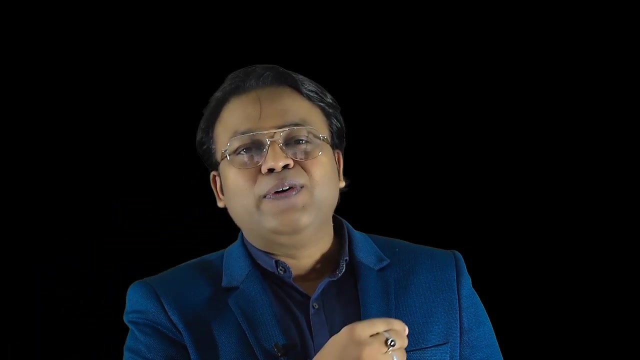 we will get the distance across the river Real world alert. Wouldn't it have been simpler to just tie a rope to the tree, climb into a boat, go across the river and measure how much rope you trailed out? In this case, it actually might be a good idea. 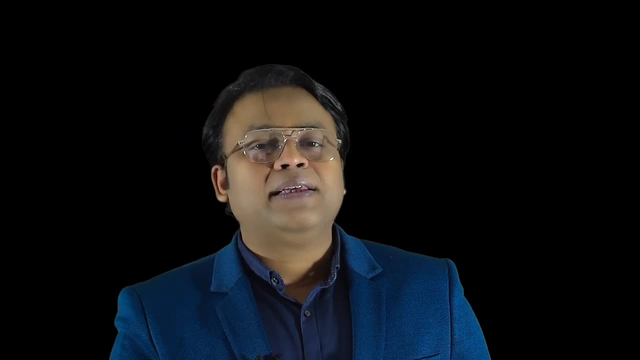 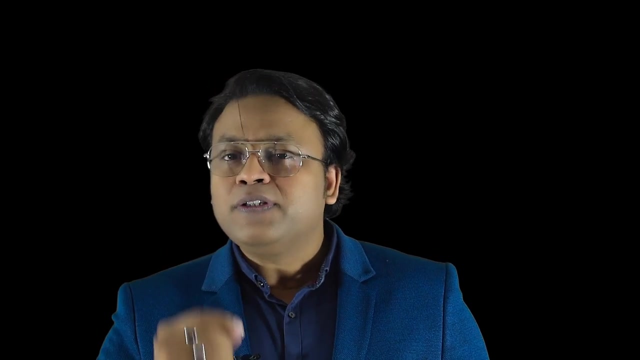 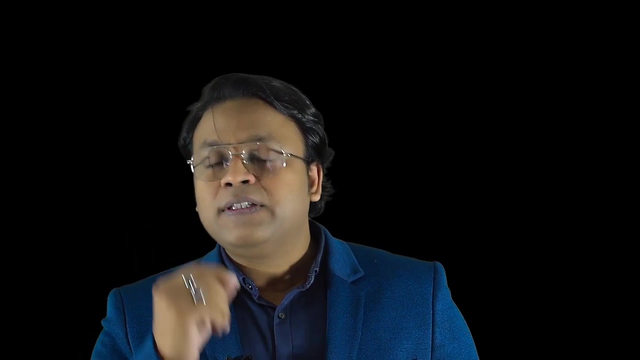 to physically cross the river to check the answer from a map. This gives us confidence that trigonometry really works. After all, sometimes real world uses a river that is too difficult to cross or a cliff too dangerous to climb. In these cases, the physical approach isn't possible. 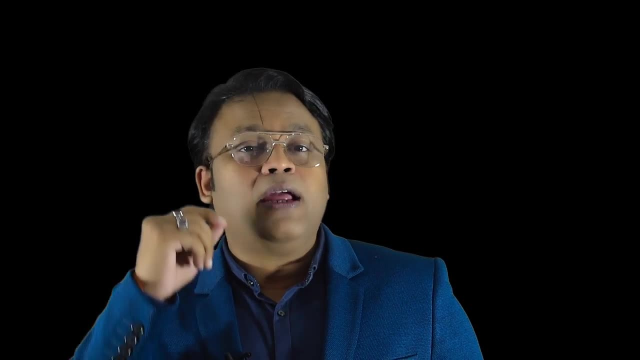 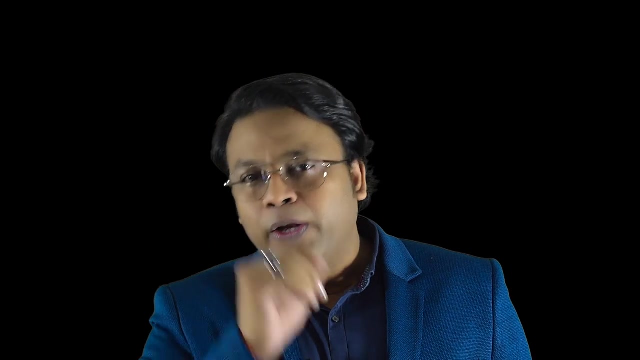 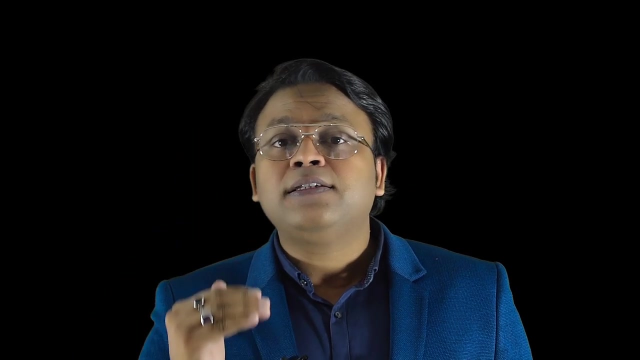 We need trigonometry, a mathematical technique we can trust, for the answers we need. Have you ever played a game called Mario? When you see him so smoothly glide over the roadblocks, he doesn't really jump straight along the Y-axis. It is a slightly curved path or a parabolic path. 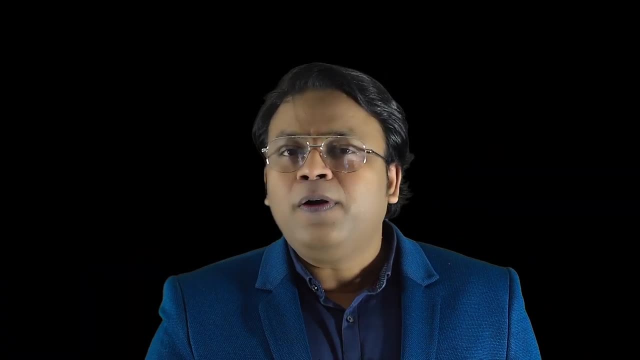 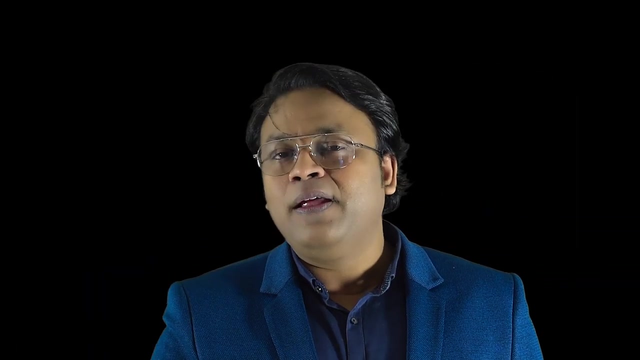 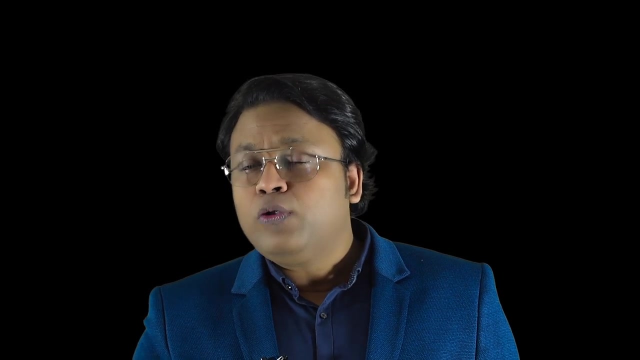 that it takes to tackle the obstacles on his way. Trigonometry helps Mario jump over these obstacles, So next time you're playing any kind of game, remember trigonometry is used over there. Flight engineers have to take in account their speed, distance and direction. 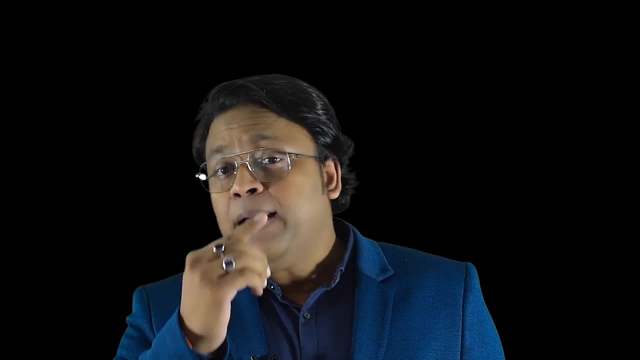 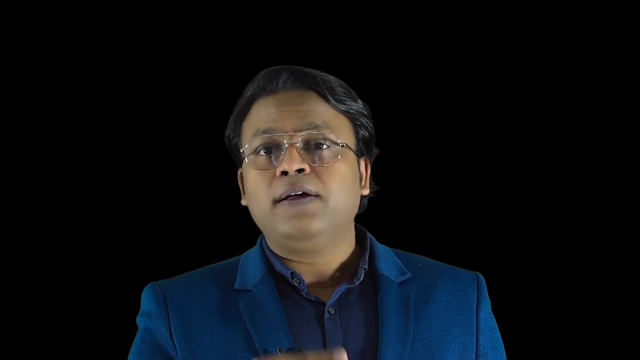 along with the speed and direction of the wind. The wind plays an important role as well. It plays an important role in how and when a plane will arrive wherever needed. This is solved using vectors to create a triangle, using trigonometry. So next time you travel by flight, 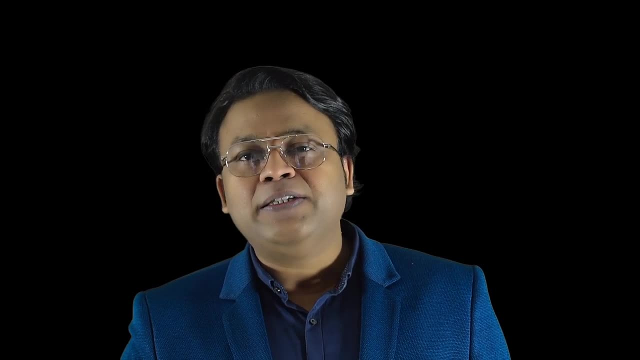 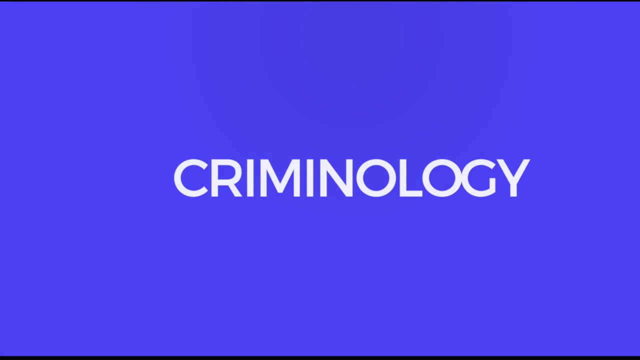 think of this, that your safety and landing of the plane highly depends upon the trajectory plotted using trigonometry. So there it is. Trigonometry is again very, very important in traveling. also In criminology, trigonometry can help to calculate. 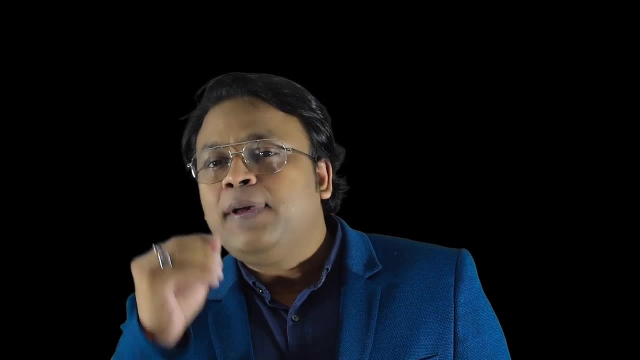 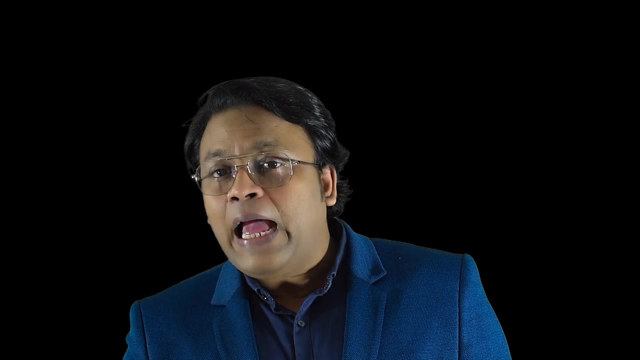 help to calculate the projectile's trajectory, to estimate what might have caused a collision in a car accident, or how did an object fall down from somewhere, or in which angle was a bullet shot. With that you can find exactly where the shooter was located. 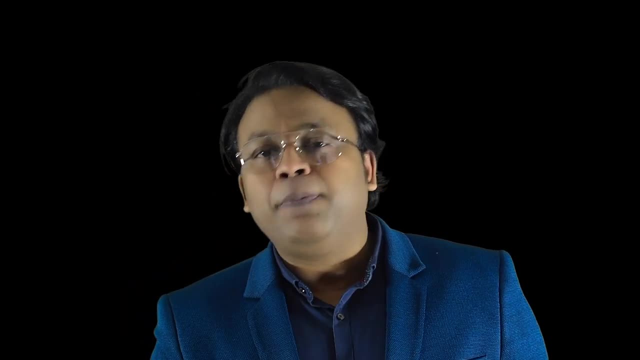 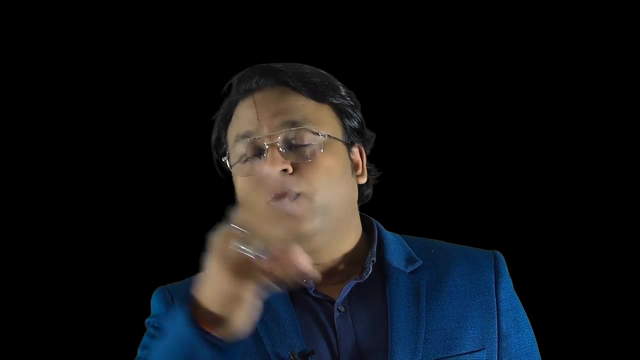 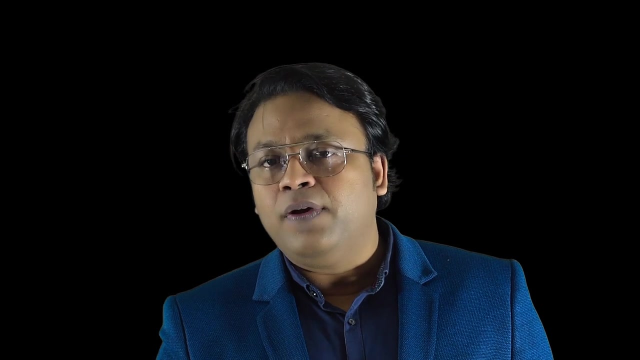 Marine biologists often use trigonometry to establish measurements, For example, to find out how light levels at different depths affect the ability of algae to photosynthesize. Also, marine biologists utilize mathematical models to measure and understand sea animals and their behavior. 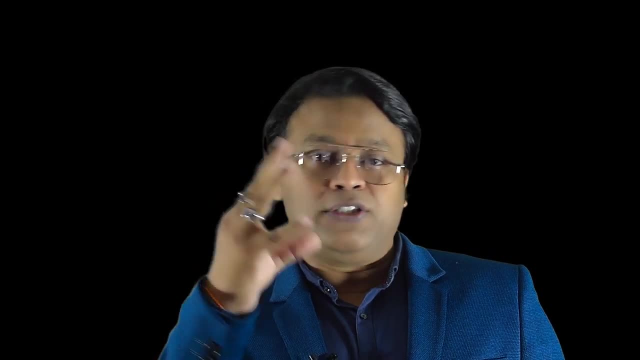 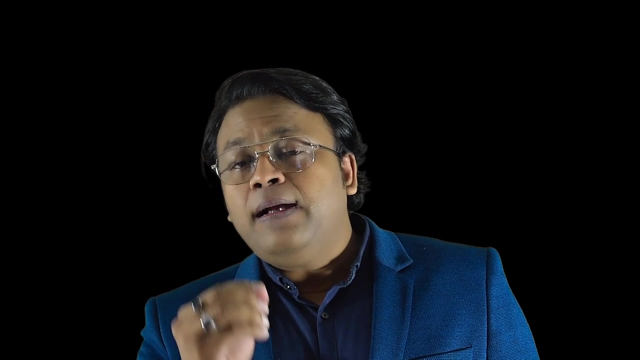 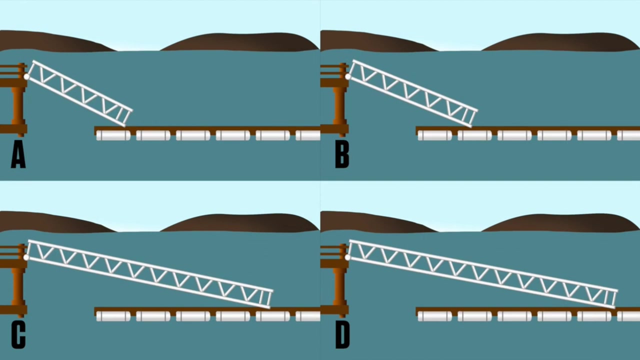 They also use trigonometry to determine the size of wild animals from a distance. In marine engineering, trigonometry is used to build and navigate marine vessels. To be more specific, trigonometry is used to design the marine ramp, which is a sloping surface to connect lower and higher level areas. 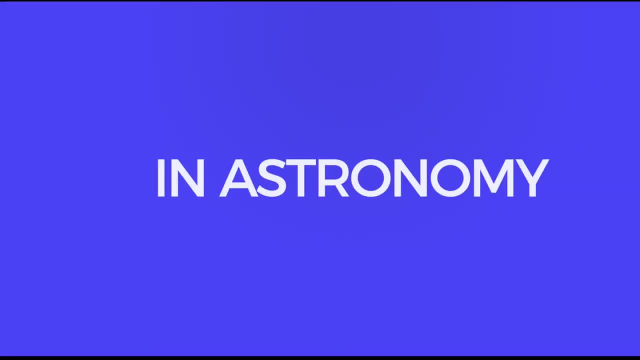 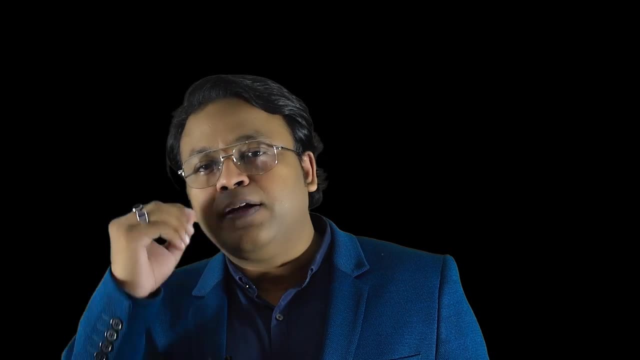 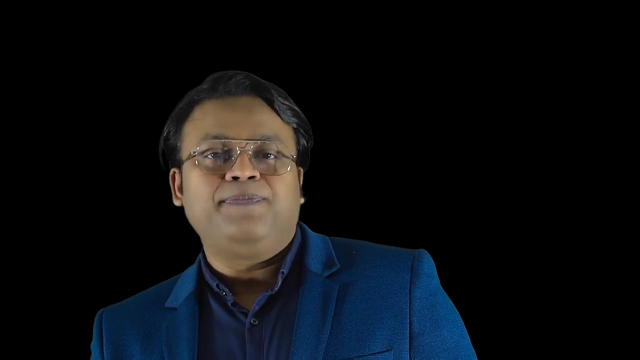 It can be a slope or even a slope. Trigonometry is widely used in astronomy. It is used in finding the distance between celestial bodies. It is used to find out the diameter and the distance between different planets. So the very important question, my friend, is that: is trigonometry important? 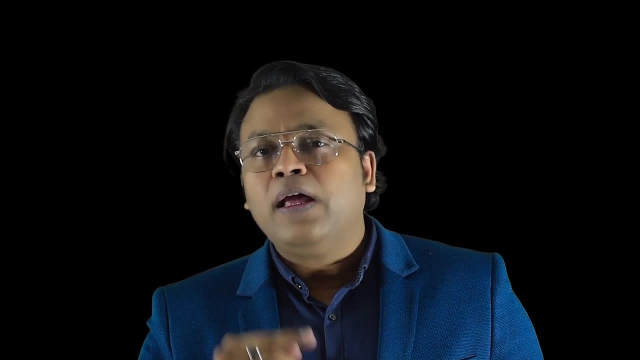 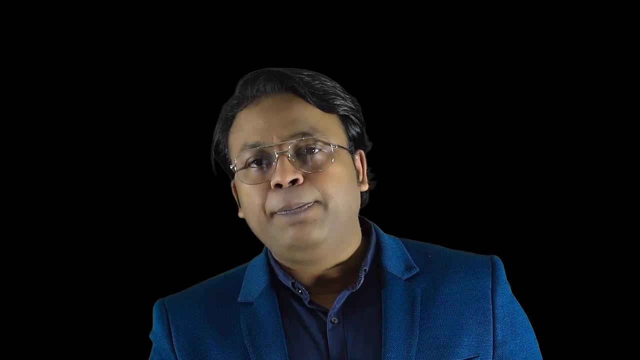 Definitely a resounding yes. Learn it, know it and use it to enhance your life. Theoretically, you could go through life completely ignorant of what trigonometry is capable of doing for you. You could have no knowledge of trigonometry or any mathematics. 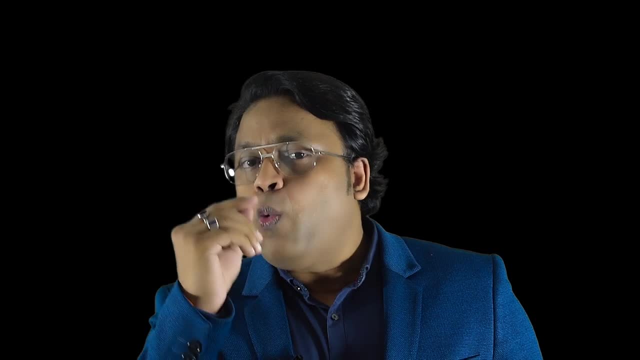 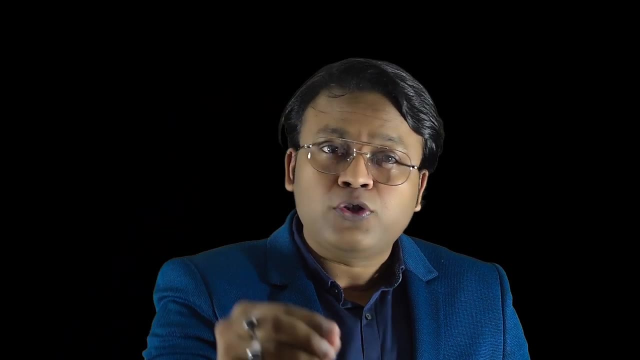 Many people do. The drawback to such a life is that one is then not able to understand the wonders that the nature has to offer. Trigonometry is very, very important. Whenever you encounter this topic in your syllabus, do learn it with a lot of passion.